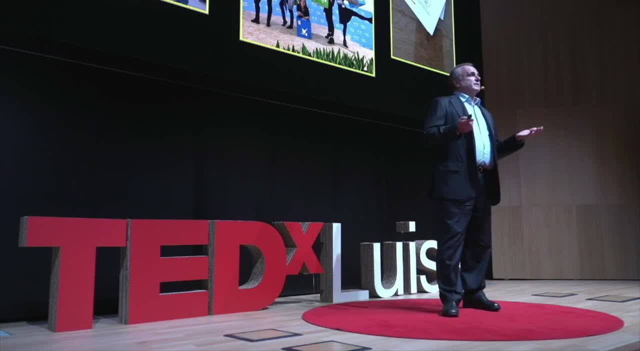 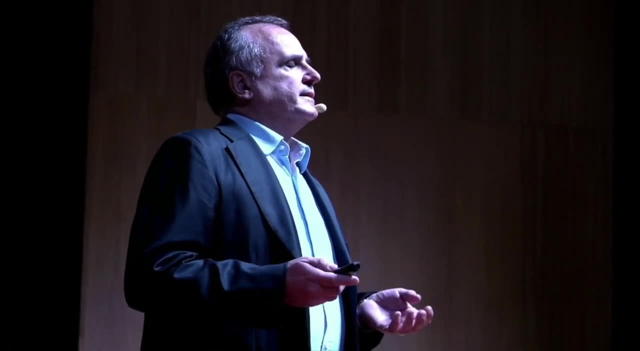 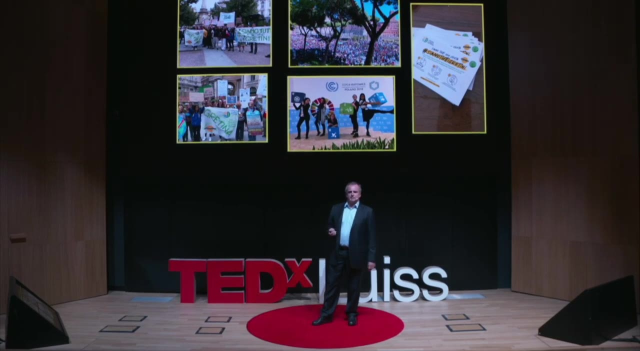 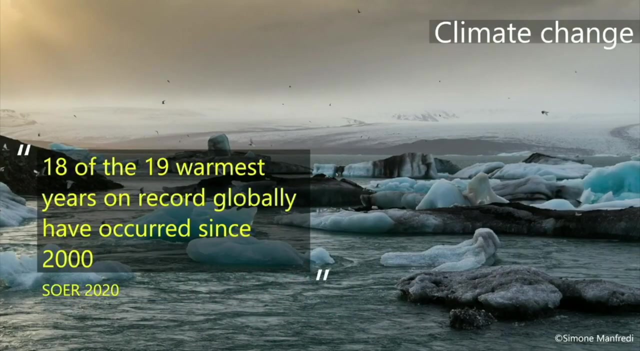 As a scientist, as a citizen and a father, I am deeply concerned about this. Years ago, I founded, with some other friends, the Italian Climate Network. It is a no-profit organization of young people to address the climate problem. Climate change is a global challenge. it is an emergency. 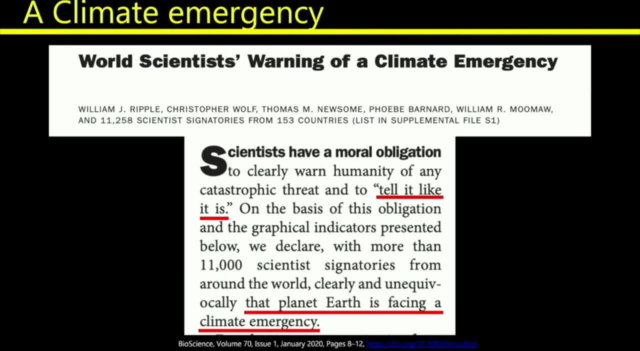 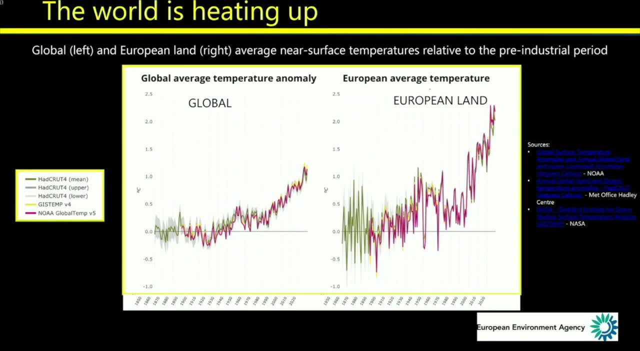 We need to listen to the science. Already, the global scientific community involved in climate science warns us about the climate emergency we are facing. The world is heating up. The global surface temperature in the last decade has gone up. The global surface temperature in the last decade has gone up. 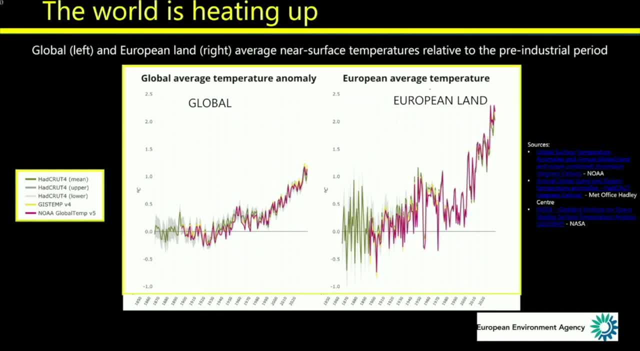 The world is heating up. The global surface temperature in the last decade has gone up. The water temperature in the last decade has gone down. The lives of the people in Europe are about 1 degree warmer than the preindustrial level. And what about Europe? 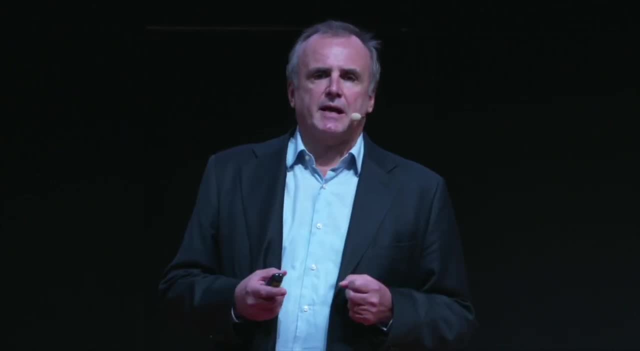 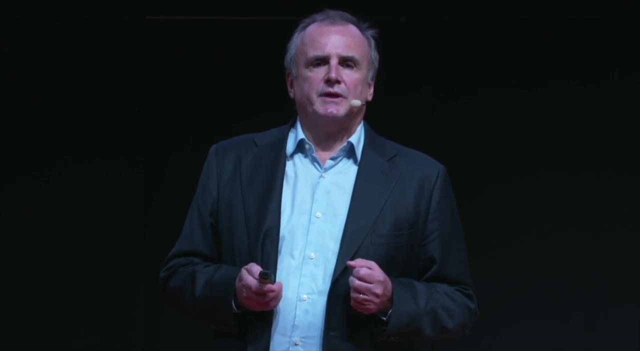 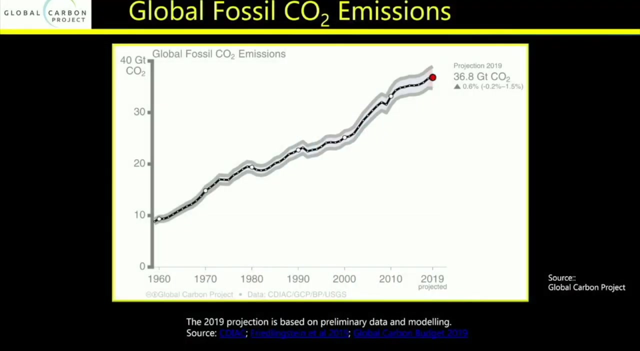 Europe's climate is not going very well. The European land temperatures have increased faster than the global ones in the same period, at almost 2°C. The global fossil fuel emissions have increased steadily in the last decade, showing recent progress decade. They show no sign of peaks. The global CO2 emissions in 2019, the last year are: 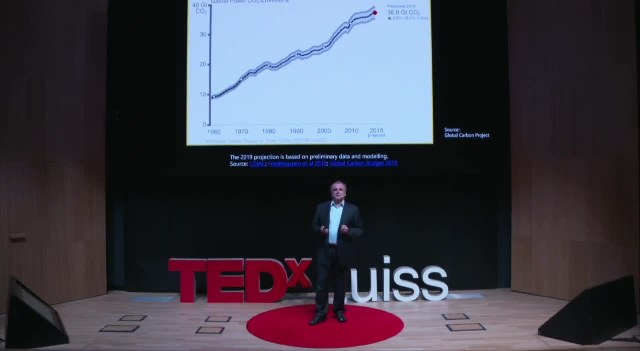 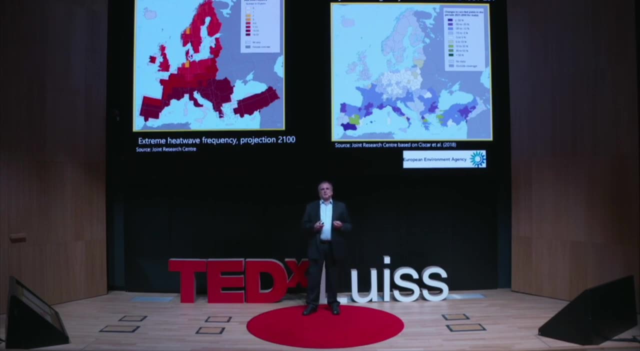 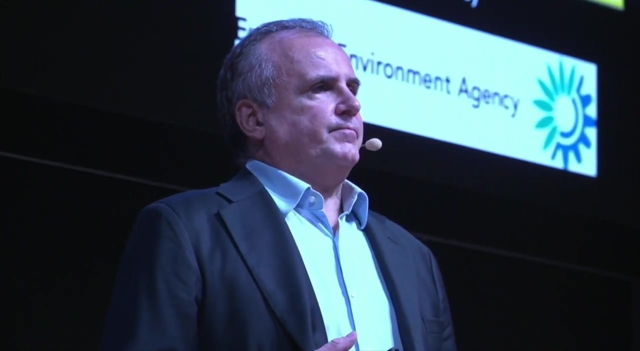 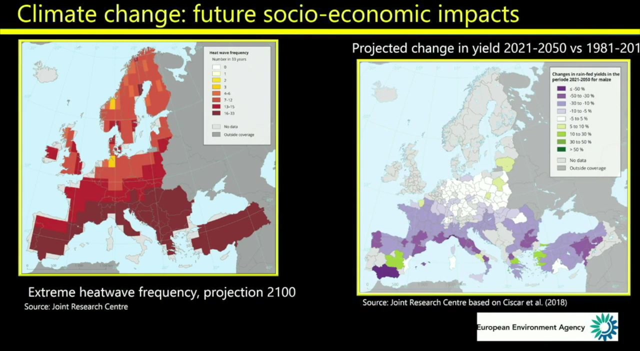 about 60% higher than 1990.. Climate change in Europe. what does it mean? Stronger climate change means stronger socio-economic impacts. in Europe. We can have more intense heat waves- heat in Europe. We can face a drop in crop production. South Europe will be the first. 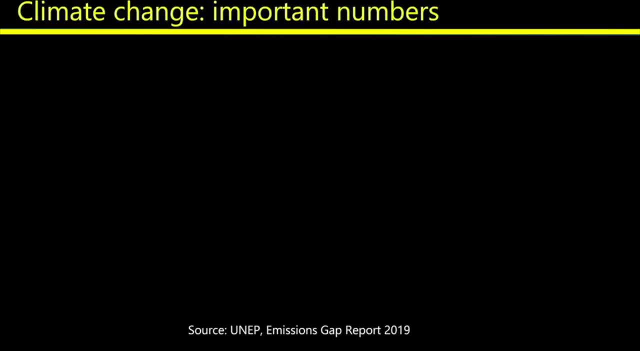 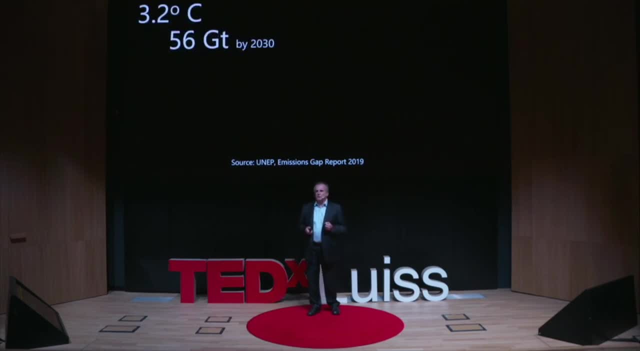 one to feel the most of this damage. About climate change, we should keep in mind some important numbers: 3.2 degrees, 56 gigatons by 2030.. With the present policy commitment in the Paris Agreement, the global temperature. 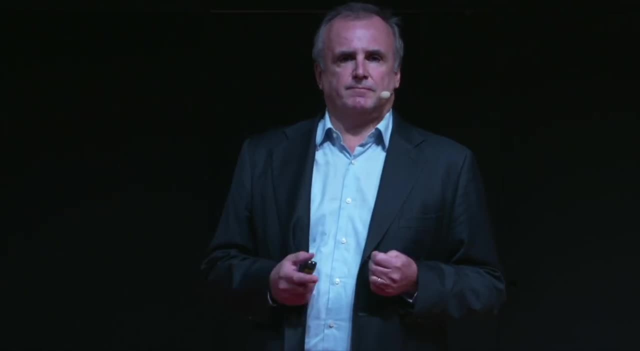 most likely will be around 3.2 degrees. The global temperature will be around 3.2 degrees. The global temperature most likely will be around 3.2 degrees. The global temperature most likely will be around 3.2 degrees. The global temperature most likely will reach 3.2 degrees this century. With these commitments in the Paris Agreement, the global emissions will reach 56 gigatons of CO2 by 2030.. 1.5 degrees, 25 gigatons, 7.6%. The objective of the Paris Agreement is to keep the increase of the global temperature. 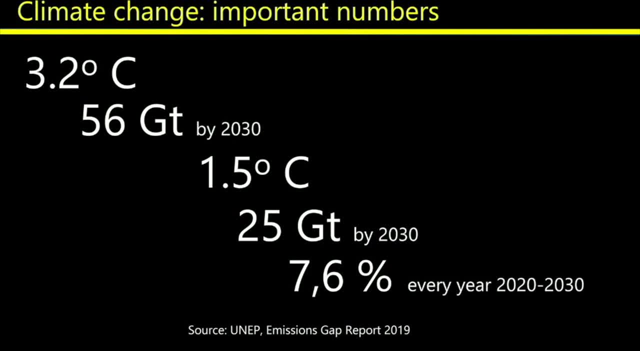 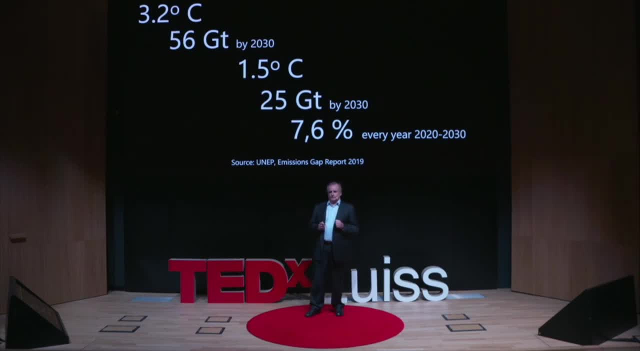 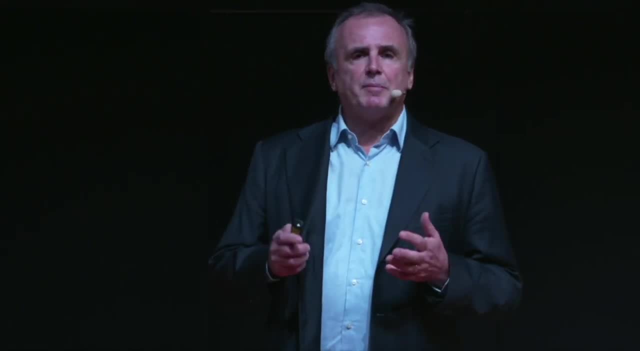 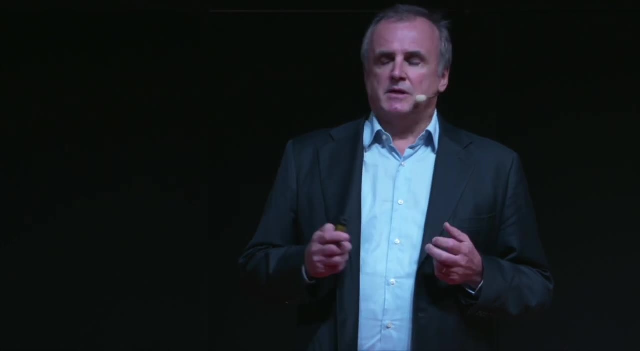 well below 2 degrees comparing with the pre-industrial level, and to make an effort to limit this increase to 1.5 degrees. To do this, science tells us something: We must drop the global CO2 emissions rapidly to reach 25 gigatons of CO2 by 2030.. The 7.6%, this last number- 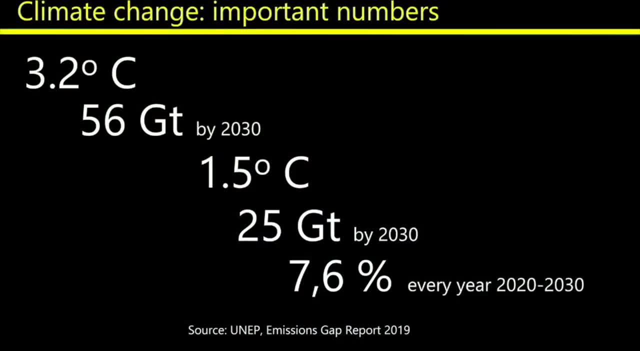 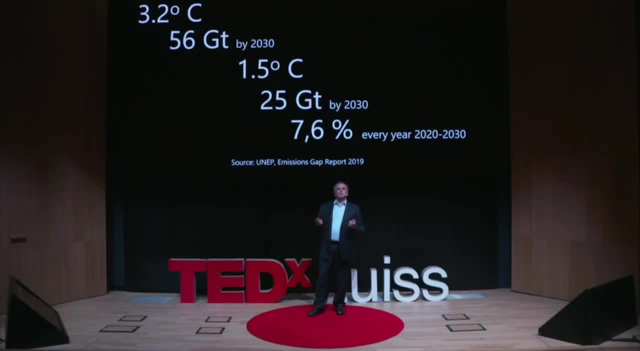 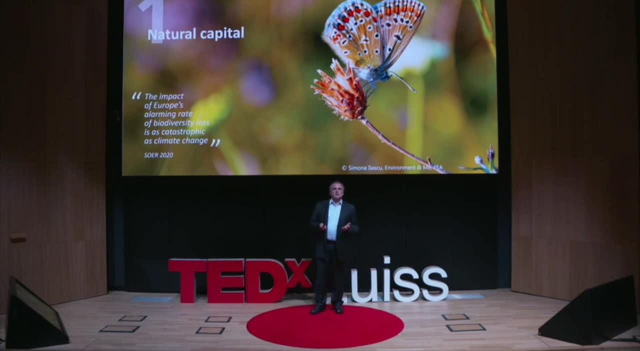 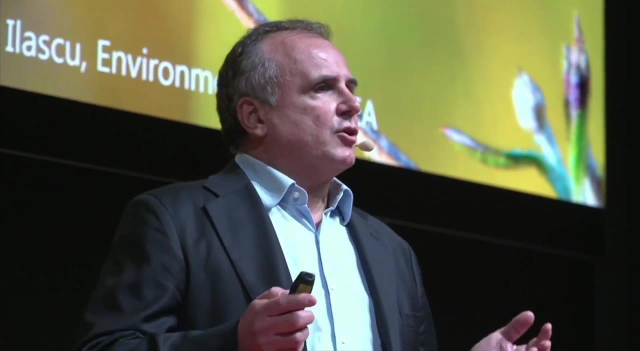 is our global solution. To do this, we must reduce our global emissions of 7.6% every year from now up to 2030.. Nature and biodiversity sustain life on Earth. The biodiversity loss and the degradation of ecosystems can have fundamental consequences on our society, the economy, the human health. 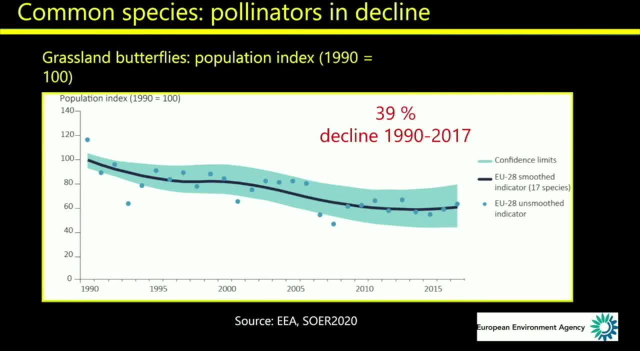 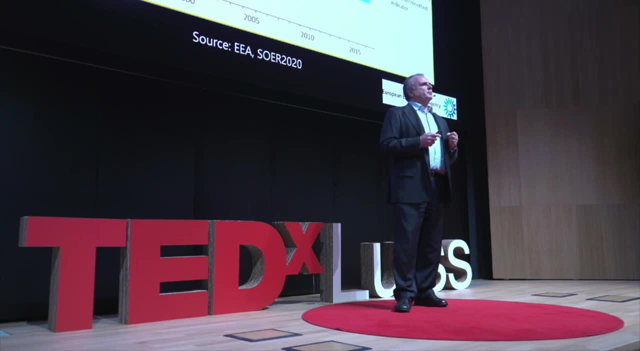 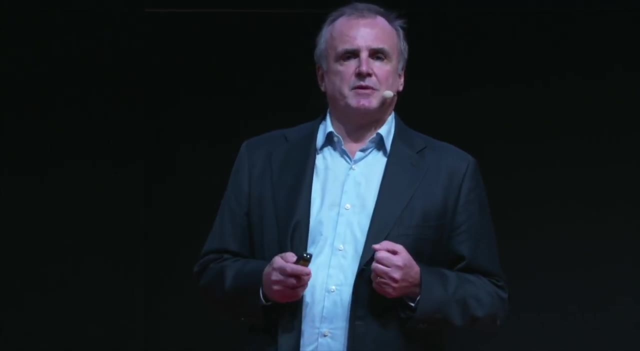 and the wellbeing and the well-being and the well-being. Europe is facing a dramatic degradation of ecosystem and the rapid loss of biodiversity. We are facing a decline in population of common birds and butterflies. Birds and butterflies are sensitive to the environmental change in the ecosystem in Europe. 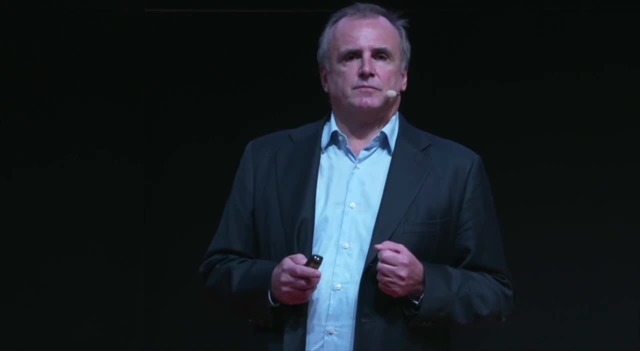 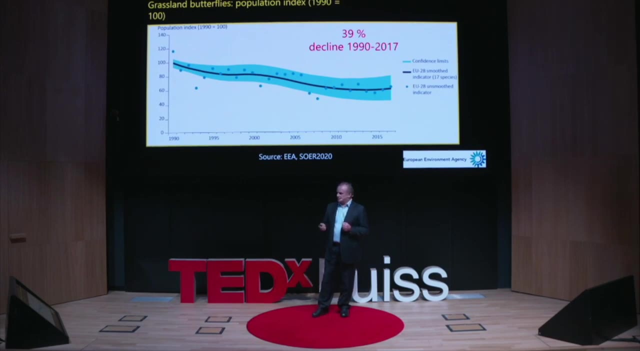 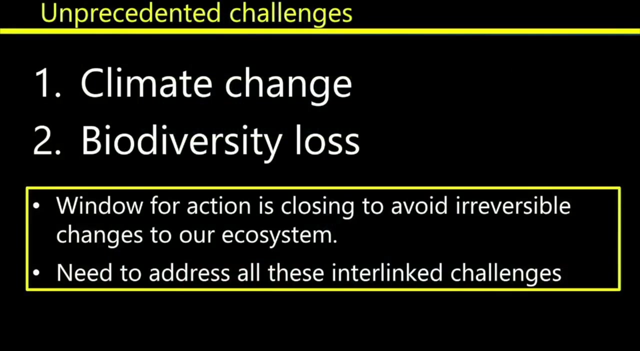 Butterflies are also a good proxy for all pollinators. These trends in population can be strong indicators of the health of the ecosystem in Europe. So we have these two challenges: climate change and biodiversity loss. We need to address this challenge together, not in a separate way. 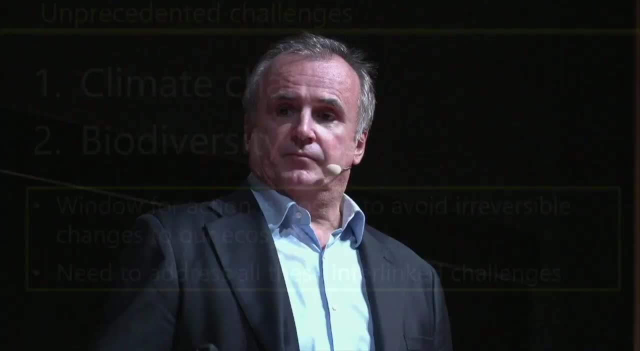 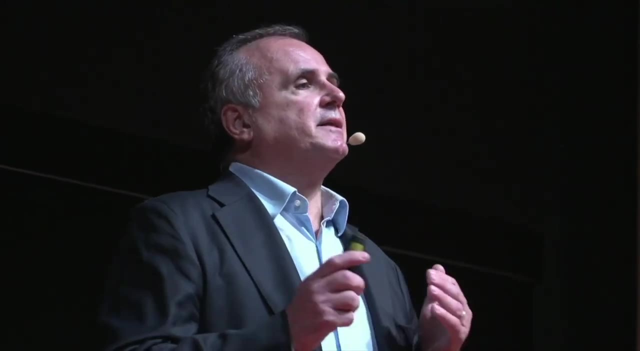 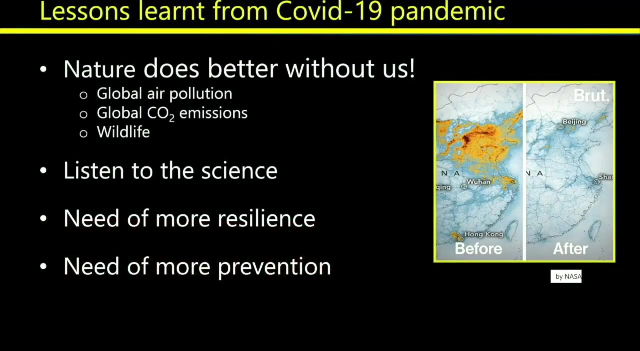 If we fail in one, we fail in both. The window for action is open. It is closing if we want to avoid irreversible change in the climate and in the ecosystem. What we learn from the COVID-19 crisis? We know very clearly the damage we produced to nature in the past. 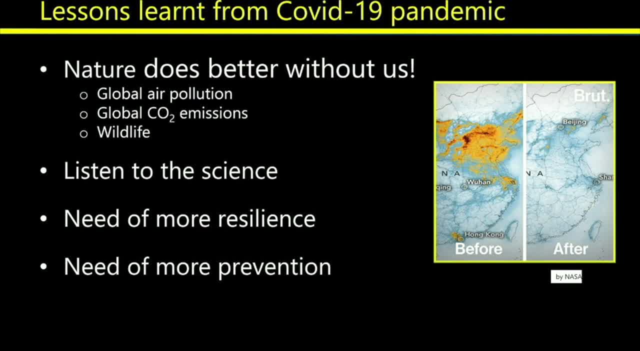 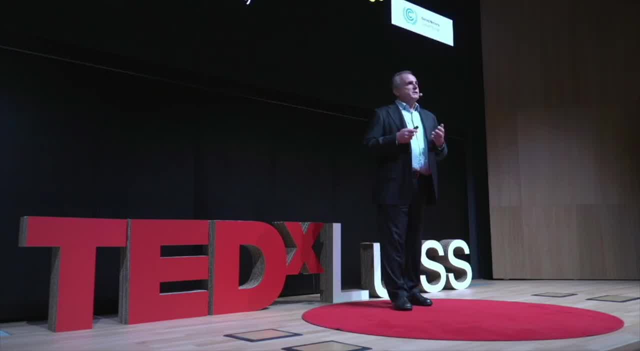 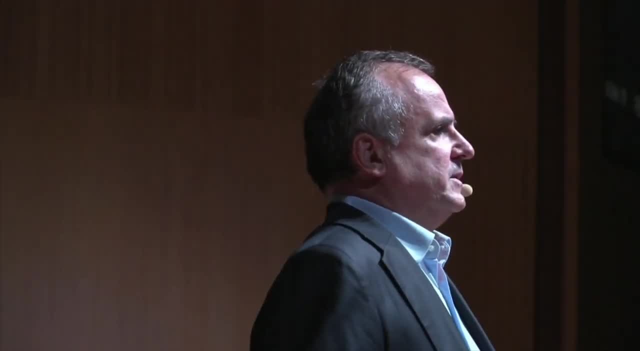 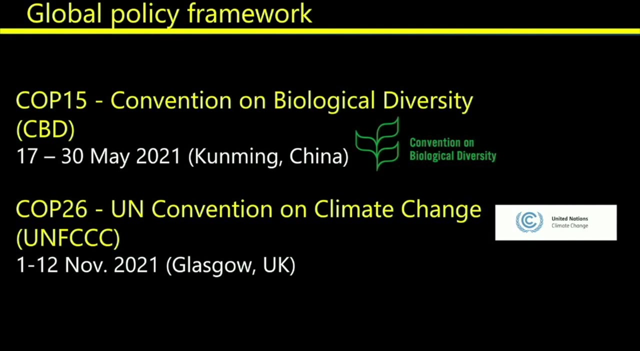 We learn that we need to listen to science. We learn we need to invest more in risk prevention and resilience. What's next? We have the opportunity to set a new course in 2021.. All the governments, the private sector, the civil society, the local authorities, the international organizations. 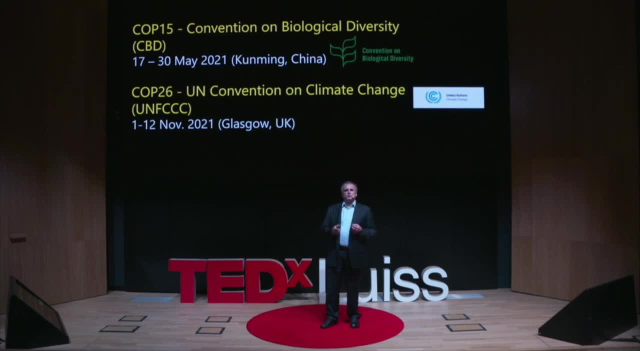 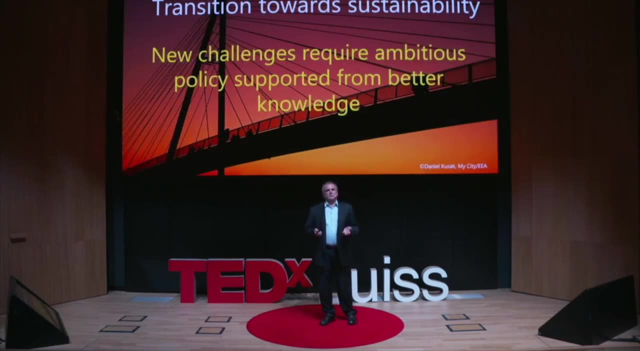 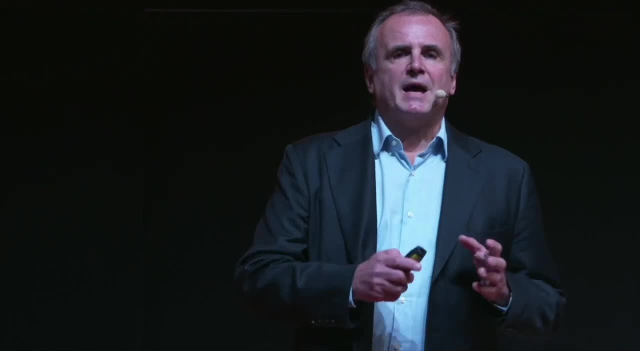 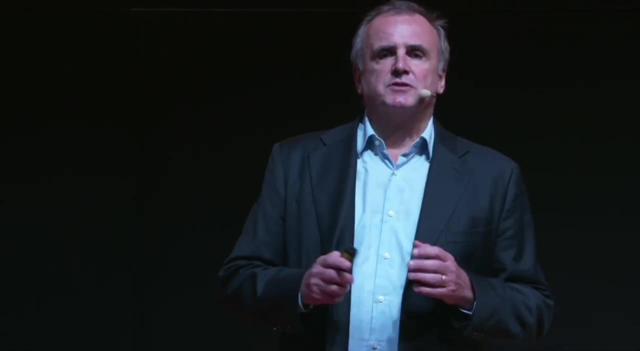 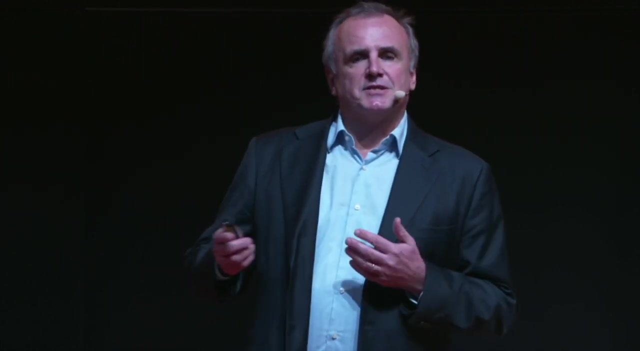 We need to think better. We need to think better. Sustainability should be our guiding principle. We must think differently. We need to transform our economy. We need to foster technology through the society. We need to build opportunities to go to a transitional to transition to ecological. 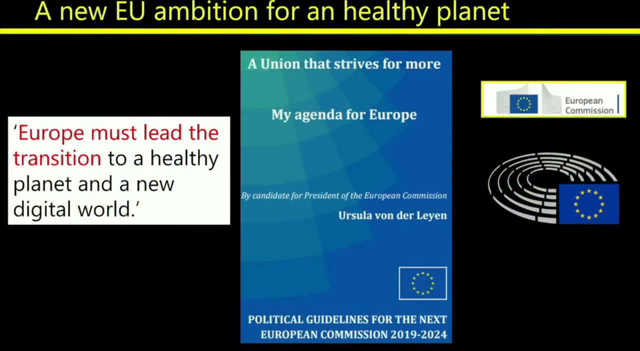 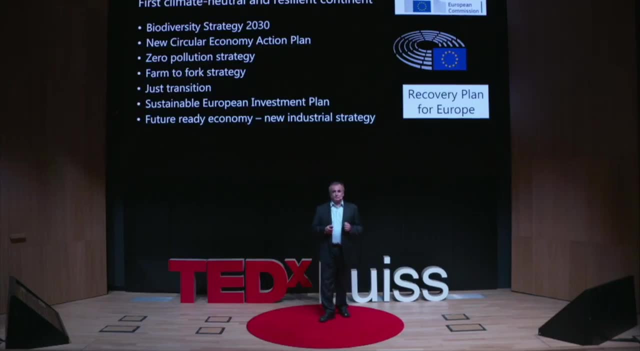 to ecological transition. Europe, European Union, has a new ambition For an healthy planet. Europe has developed a new transformative policy framework. This framework is the European Green Deal. The objective is to have, by 2050, a climate neutral and resilient Europe. 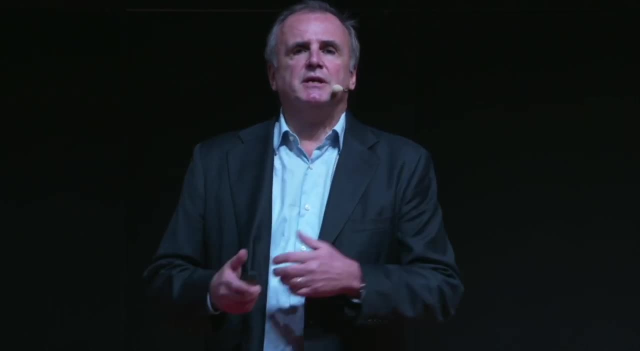 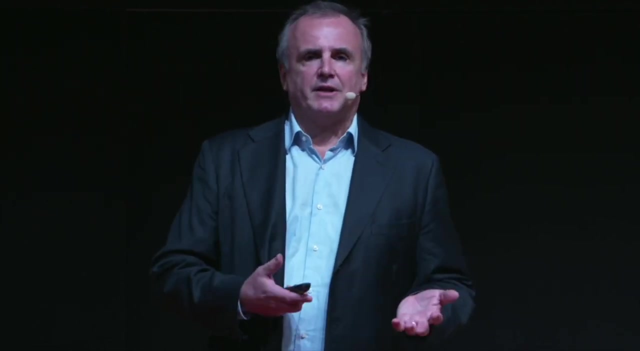 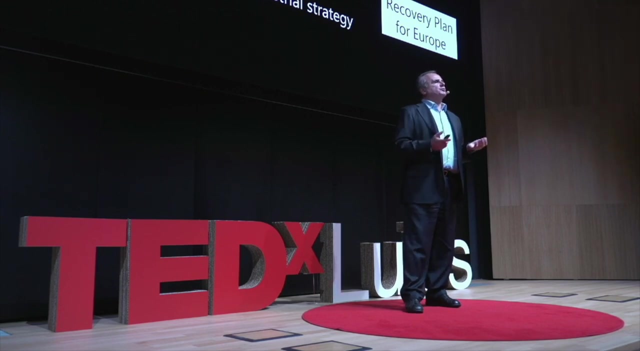 It is a roadmap. It means change in European policy plans and action. New strategy, New plans, New action, New action For biodiversity, For climate change, For climate change For pollution, For industrial development, For industrial development For many socio-economic sectors of the European society. 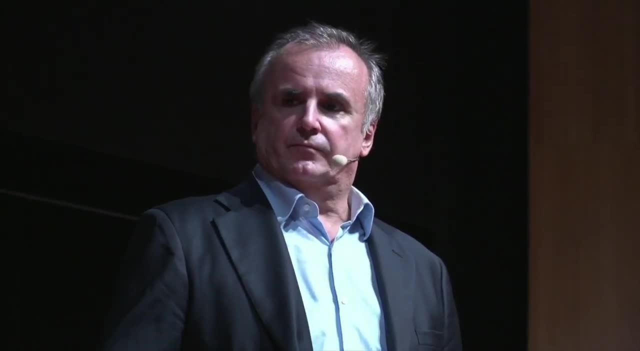 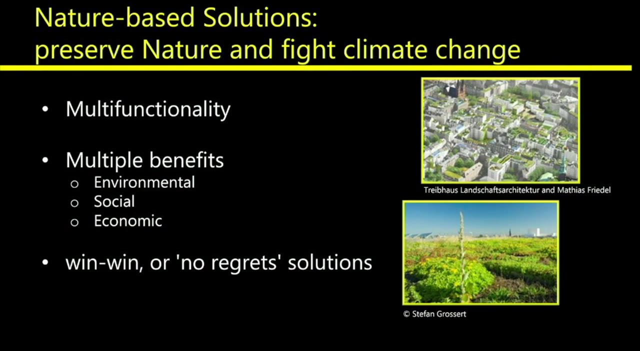 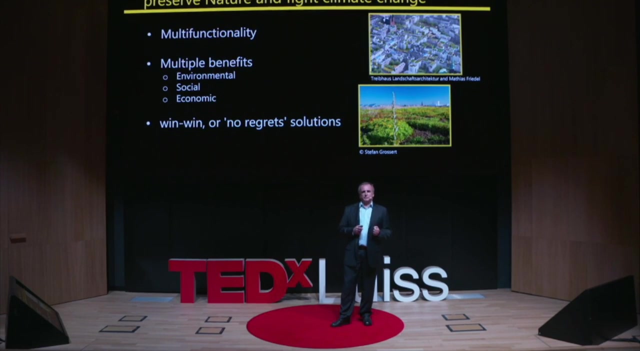 For many socio-economic sectors of the European society. Natural-based solutions and green infrastructure are among the solutions to make this European Green Deal real. They work with nature. They preserve nature. They fight climate change, climate change. They fight climate change through climate change adaptation and mitigation. 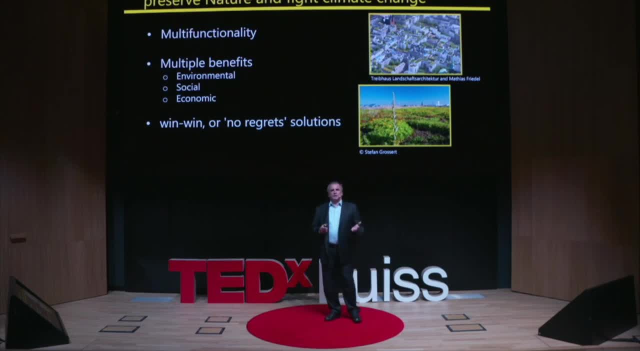 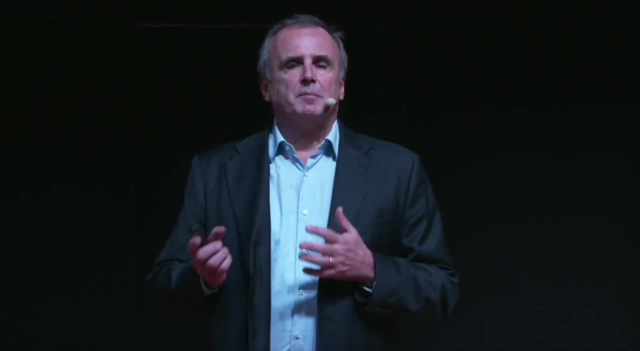 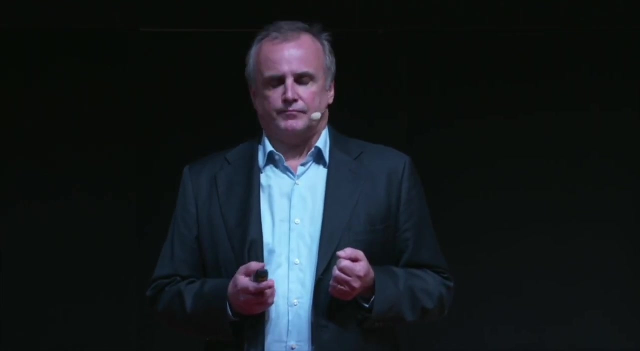 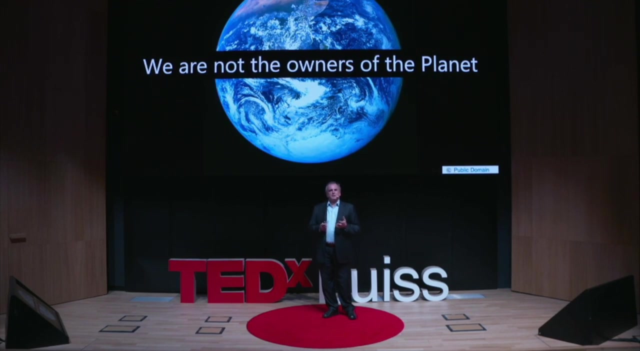 They also provide multiple benefits: ecological, socio-economic benefits. The natural-based solutions benefit biodiversity and they support the delivery of many ecosystem services. So today I present you evidence of these two global challenges: the challenge of climate change and the challenge of biodiversity loss. I show you some European solutions which will